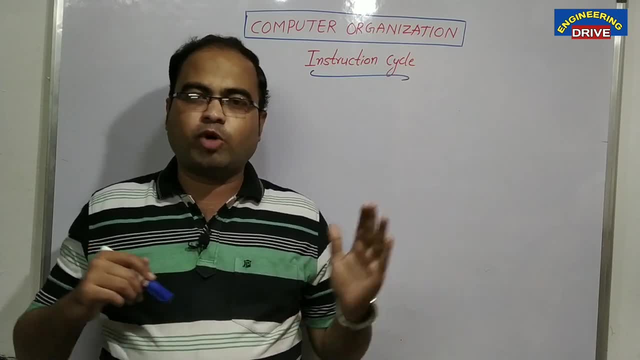 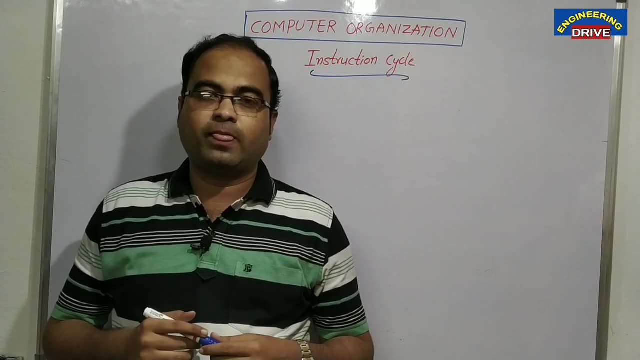 of computer organization. in my channel you can find in a proper order. Okay, so you know that the last topic which I have discussed in computer organization is about types of memories. Okay, that is my part number six. Now let us go ahead. one more step. now Let us start. 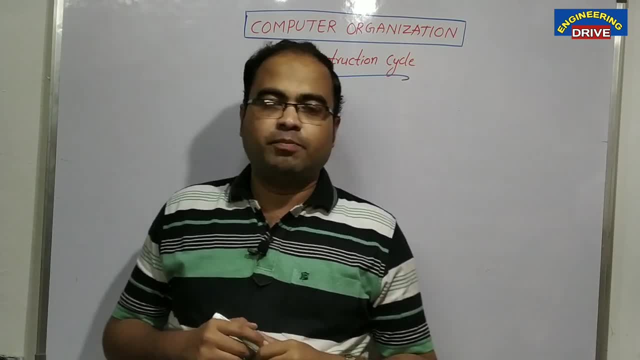 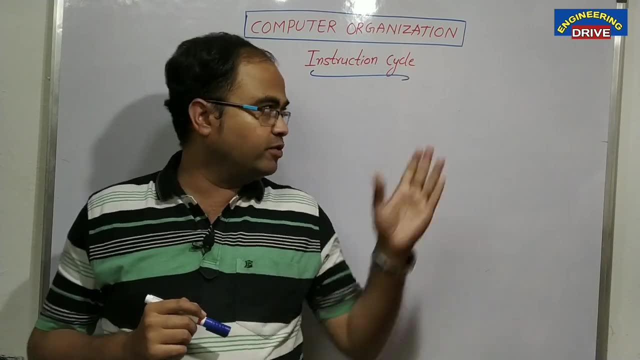 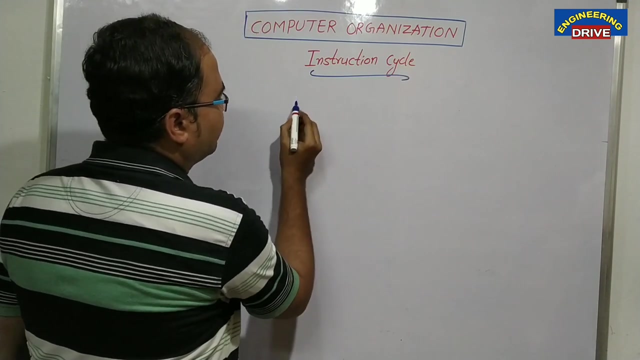 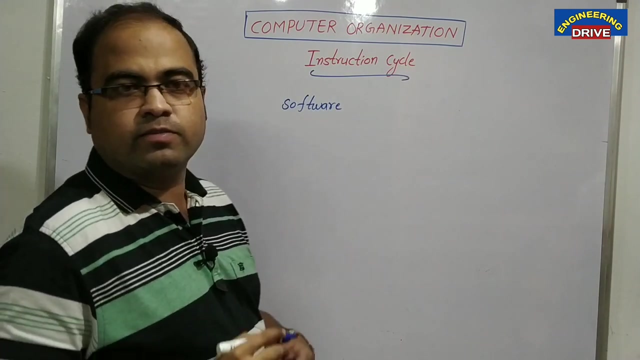 and let us discuss about what is instruction cycle, Because instruction is also a very, very important part of any computer. Okay, what is instruction? First of all, we should know, then we can discuss what is instruction cycle. Okay, so, my dear students, we know that. what is the definition of a software? Okay, what is a software? 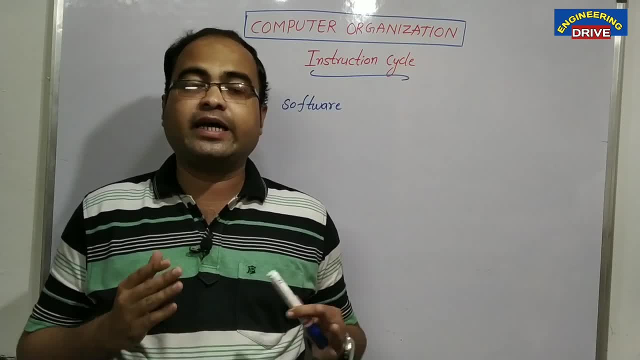 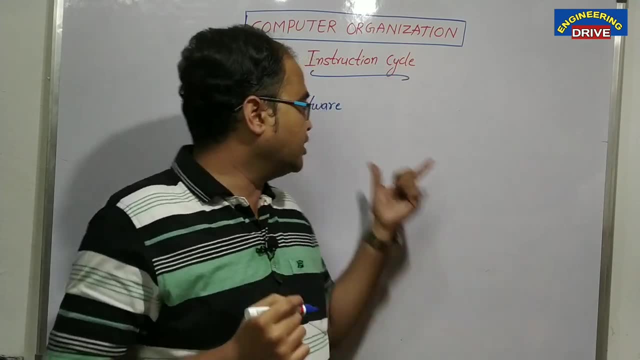 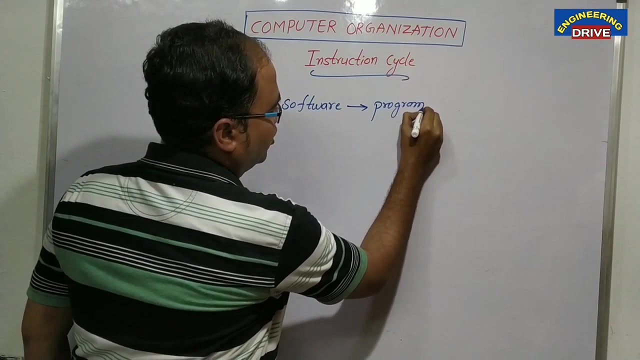 So what is the definition of software? A software is defined as a collection of programs. We can say that in our computer software is available. We can say that in our smartphone software is available. A software is nothing but collection of programs. Okay, a software is nothing but collection of. 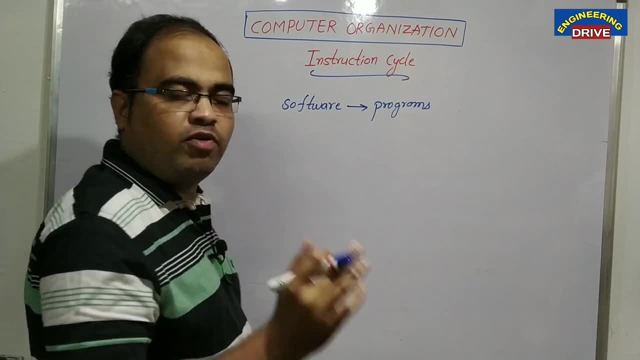 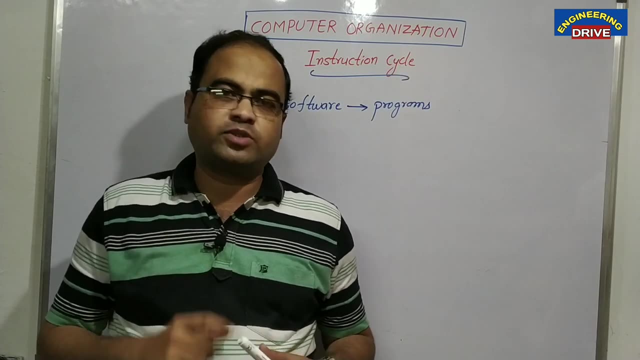 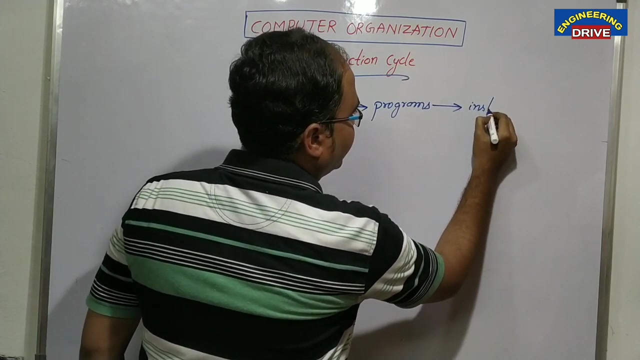 programs, Then what are programs actually? If you want to develop a software indirectly, we want to develop programs. Okay, then what is each program stands for? Again, if we go in some more, some more depth, each program is a set of instructions. 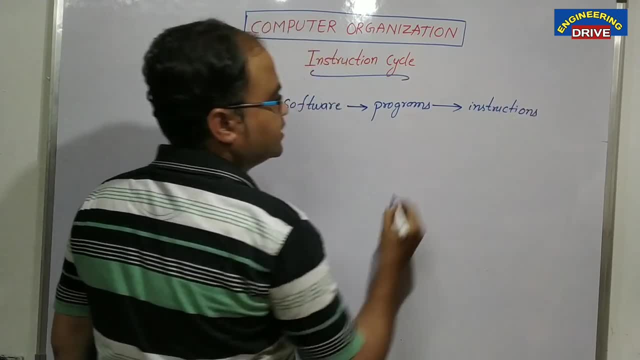 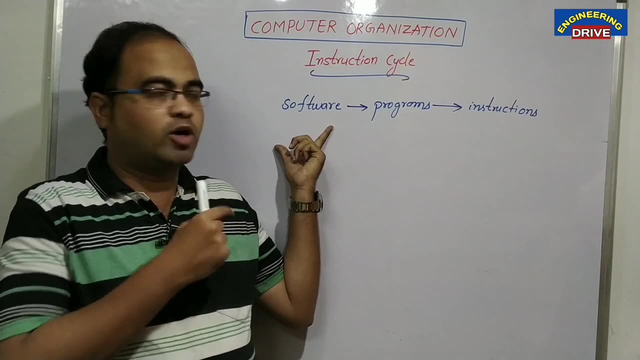 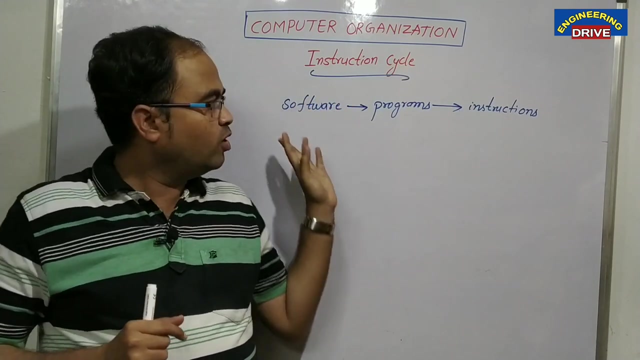 Each program is a set of instructions. So this hierarchy, we should know: first, What warfare are, what is software? Software is the collection of programs. Then what is a program? a program, each program is a set of instructions, which means what is the smallest entity out of these three? instruction is a smallest entity which? 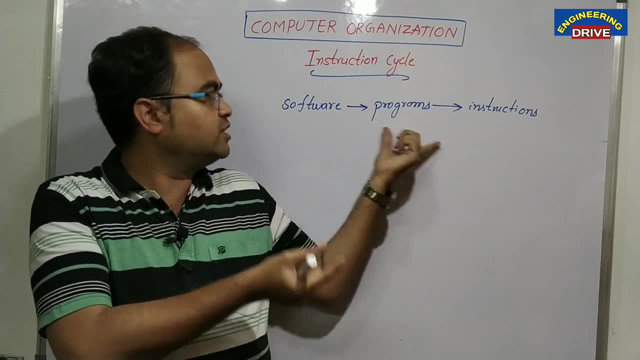 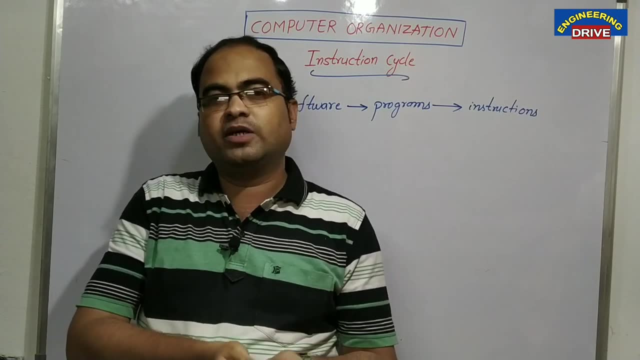 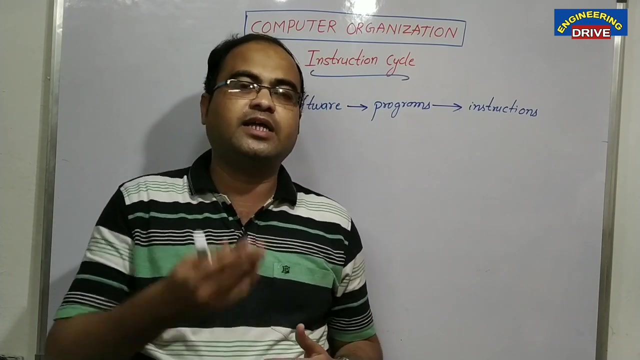 is available inside a program again is: program is a entity which is available inside software. so what software engineers are doing nowadays? software engineers are not only developing software. it indirectly means that they are developing programs. if they are developing programs indirectly, it means that they are developing instructions. okay, suppose i want to develop one software. i need to start. 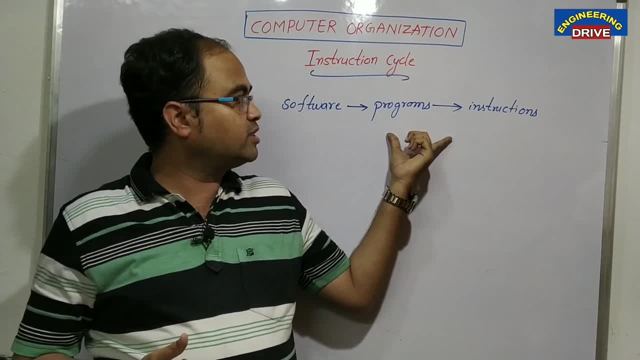 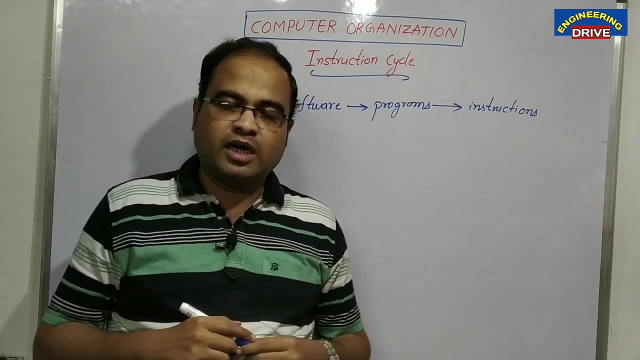 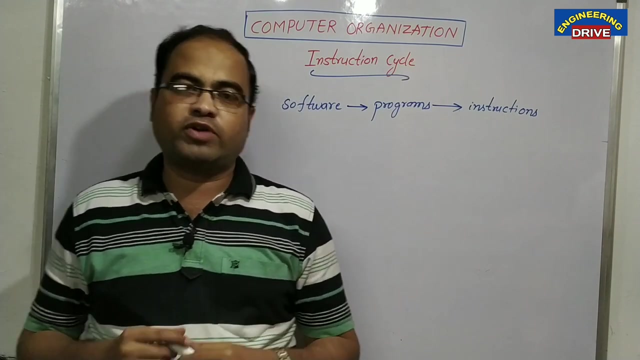 from scratch. i need to write instructions first, then those instructions forms a single program. if i write multiple programs, those multiple programs forms a software. okay, now, if my computer is running a software, what is the meaning inside this? generally we can use this word: i am running a software in my computer. i am running a software in my mobile phone. it means that programs are. 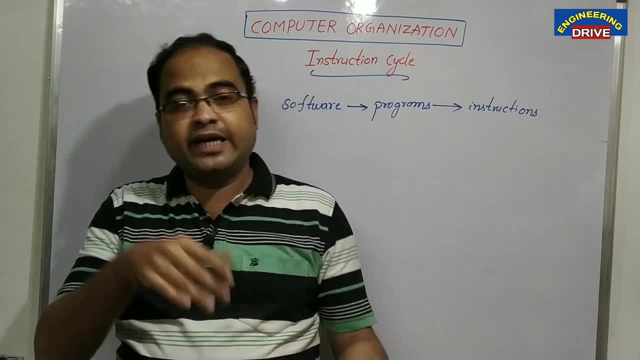 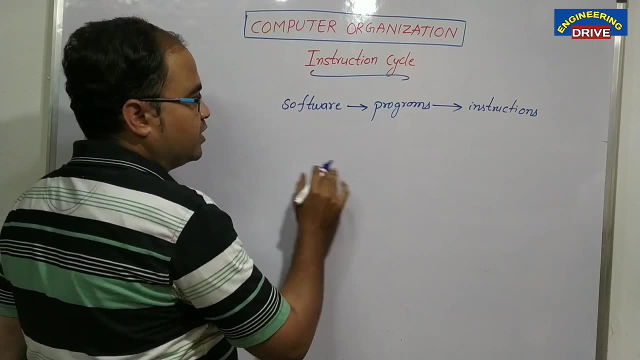 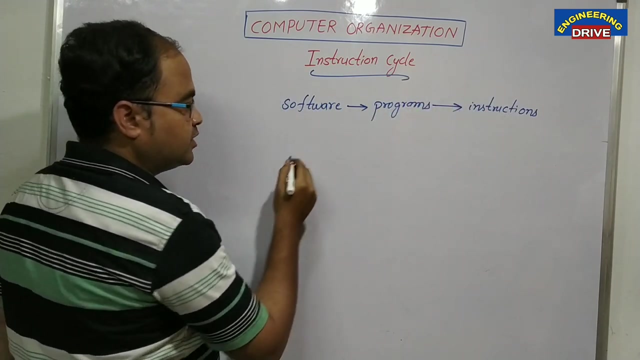 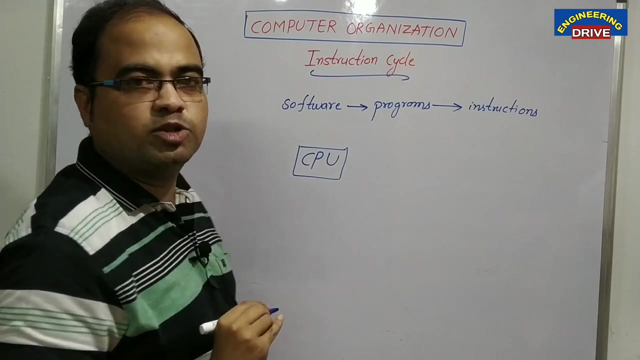 been running in the system. okay. programs means, indirectly, instructions are running inside the system. okay, which means who is responsible to execute our, our entire software? who is responsible to execute our entire programs? who is responsible to for the execution of instructions? the entire work of our computer is will be done by our cpu. what is cpu stands for central processing unit. 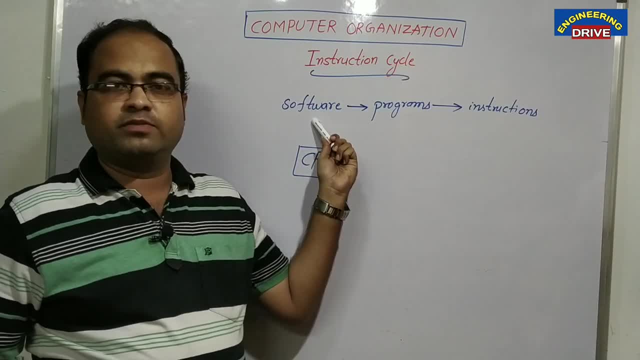 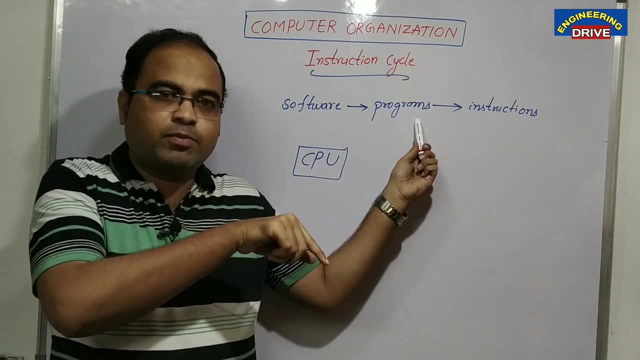 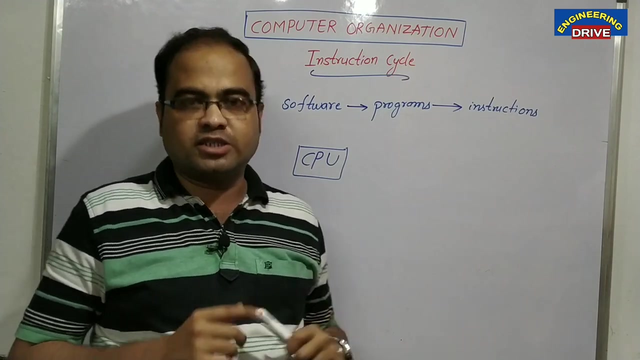 cpu is mainly responsible to run the software. if cpu is running the software indirectly, it means that cpu is running multiple programs. if cpu is running a single program, it means that cpu is running set of instructions. okay, how our cpu will execute these instructions. our cpu will execute the instruction in stepwise. 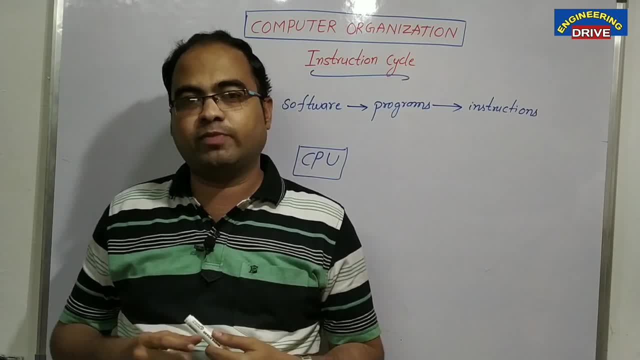 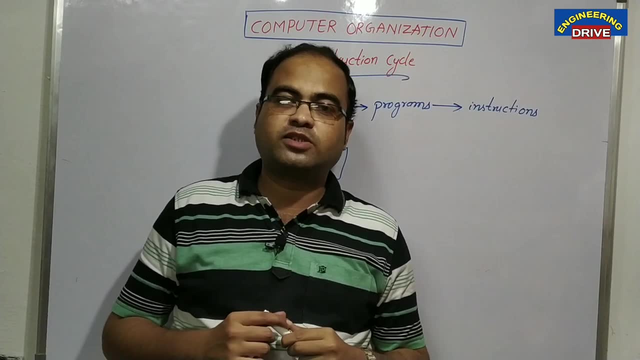 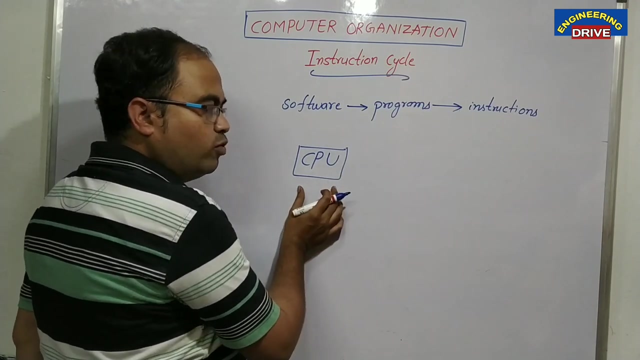 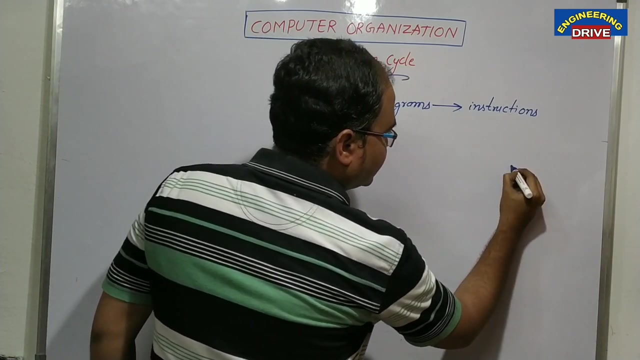 manner. however, cpu will execute the instruction in a stepwise manner. we call those collection of steps as instruction cycle. what we call those collections of steps instruction cycle. let me clear this one. okay, what is the first step our cpu will do? let us say: this is my computer and this is my hard disk. and from hard disk, let us say: this is my hard. 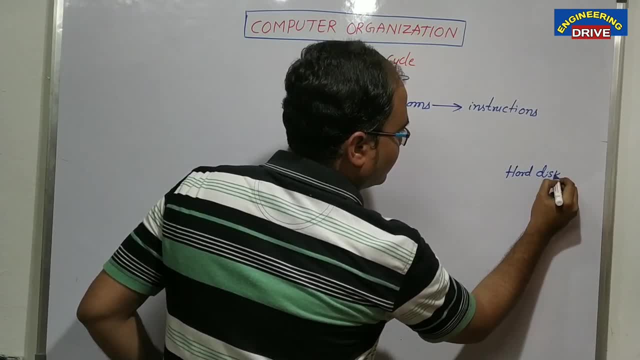 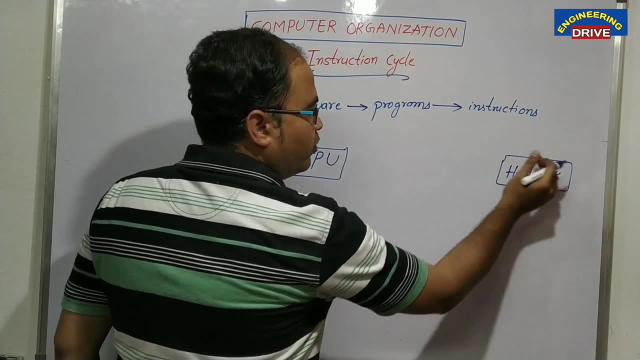 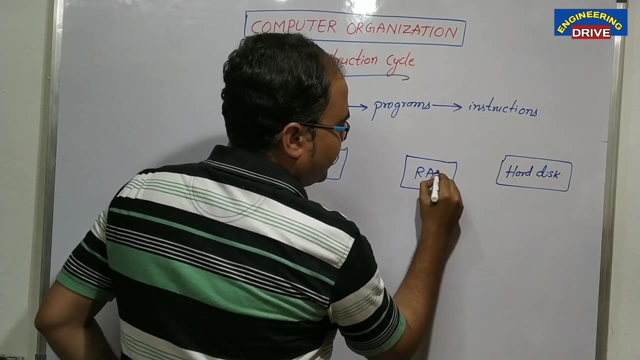 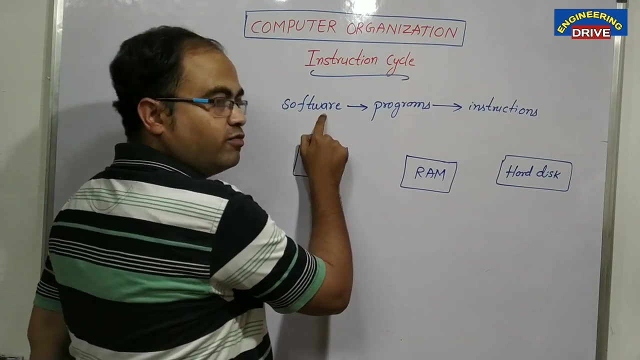 disk. okay, if our cpu want to execute one program. what happened? cpu will take the data from hard disk, and from hard disk the data is copied into primary memory, or we can say main memory or random access memory. so what happened? where we will install our software first? once we install our software, it is stored in hard disk first. 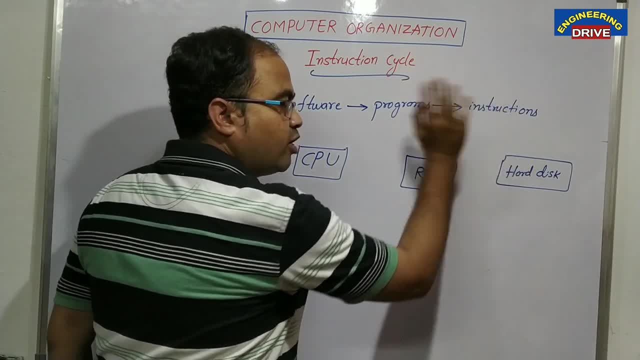 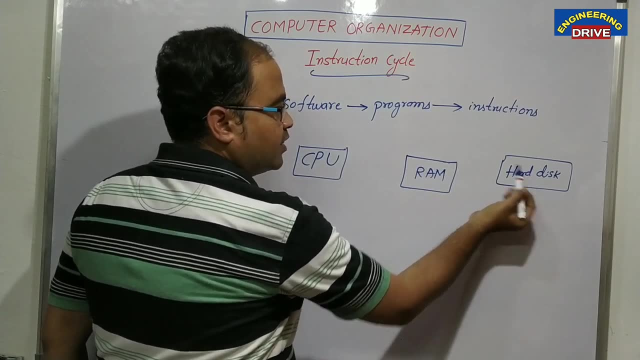 so what is? software means collection of programs. each program is a set of instruction. this one we should not forget. okay, my dear students, so what happened when we install software? let us say the software size is the software which i have installed is, let us say, 500 megabytes. 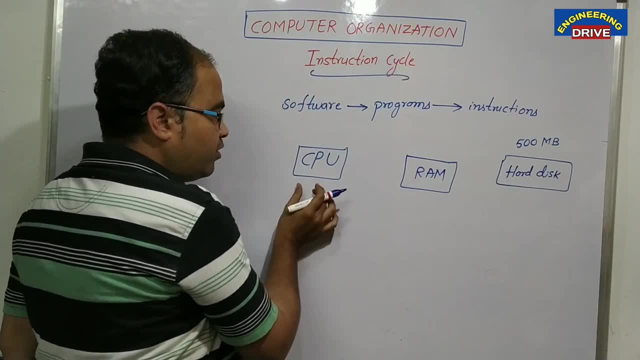 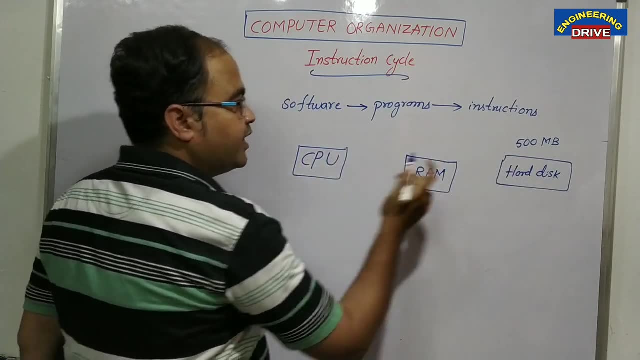 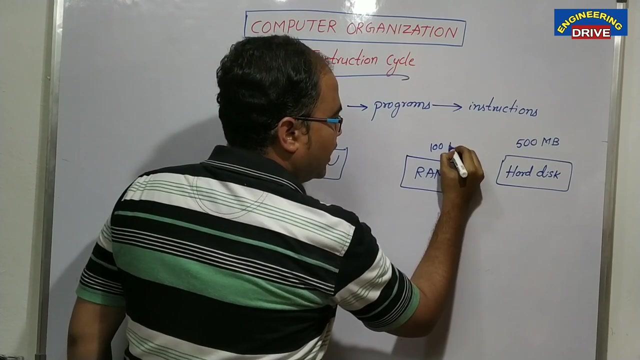 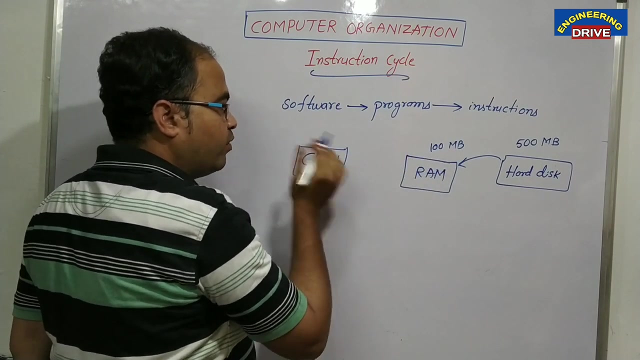 the size of my software is 500 mb. so what my cpu will do, it will take it. it won't take that entire 500 mb from the hard disk. it will take only the necessary part of that 500 mb. let us say it will take only 100 mb. only 100 mb will be stored in ram and from that 100 mb what our cpu will do. 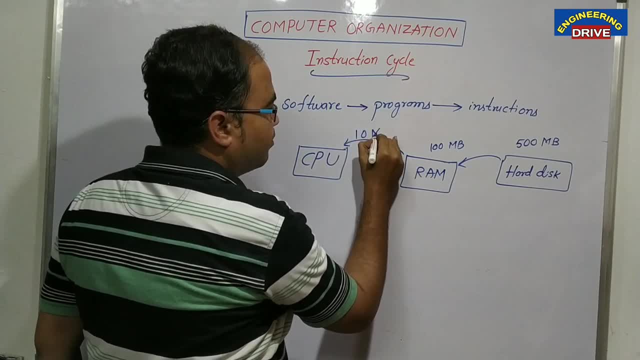 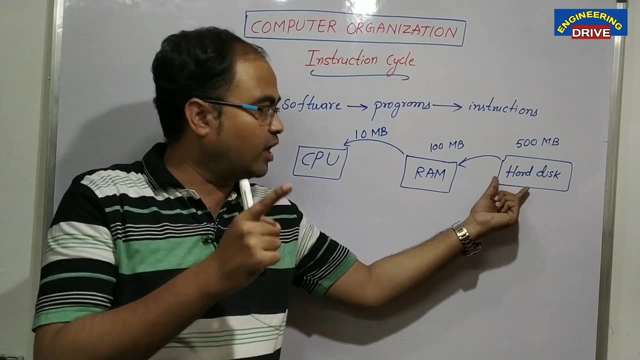 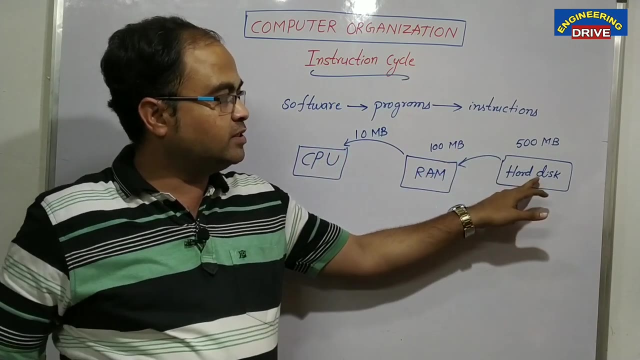 it will take only the necessary part, let us say 10 mb, which means it will take the first instruction from the hard disk and it will be copied into ram. again from ram it will be copied into cpu in a decreasing size manner, which means the size of 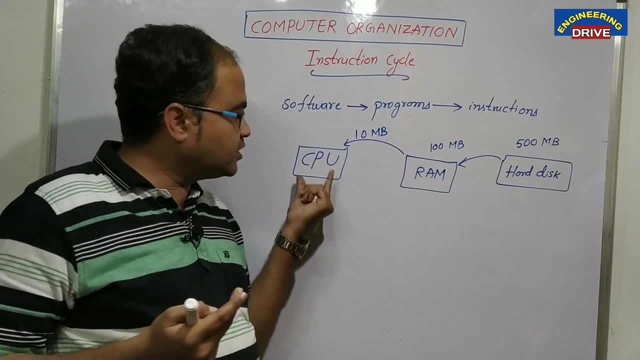 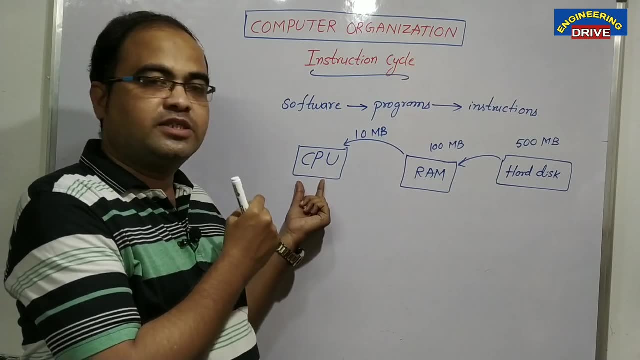 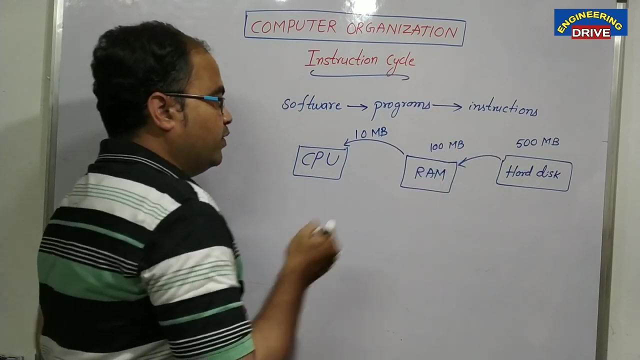 the hard disk is larger. next larger size is ram and next one cpu, which is the very smallest memory in this one. cpu is the cpu is a entity which is very small in size. next is larger one ram. more larger one hard disk. okay, so what our cpu will do? it will take the instruction from hard disk to ram and from ram. 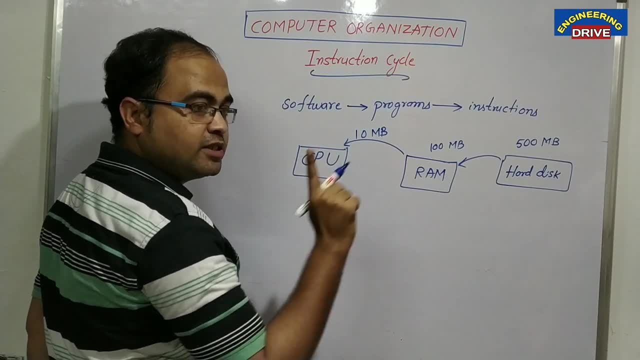 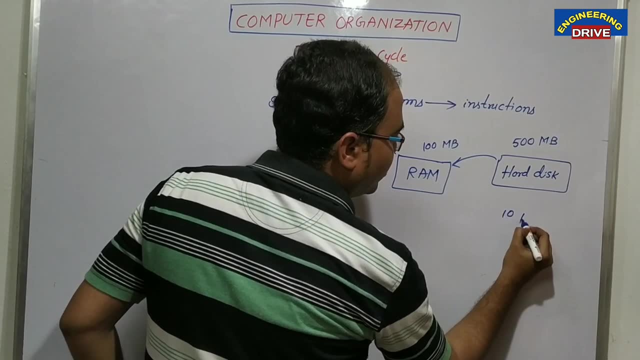 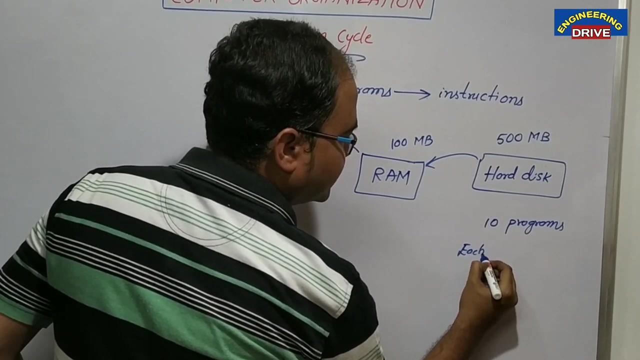 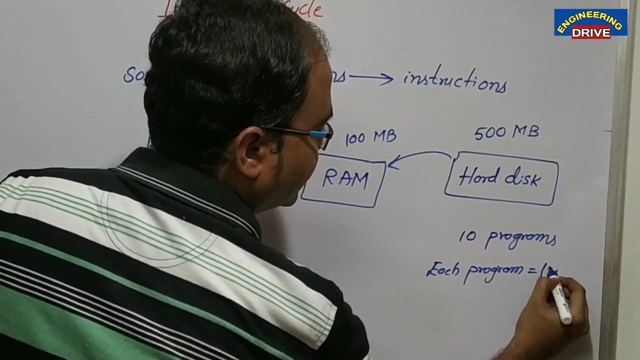 it will take to itself and it will execute one instruction. how many instructions? only one instruction. let us say: my software contains 10 programs. how many programs? 10 programs, again, my each program. let us say: my each program contains one in. let us say 10 instructions. sorry, how many instructions. 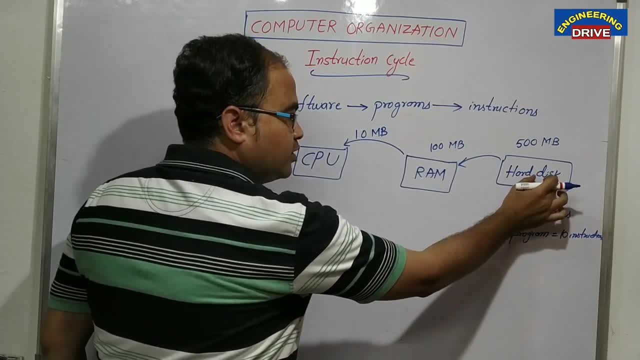 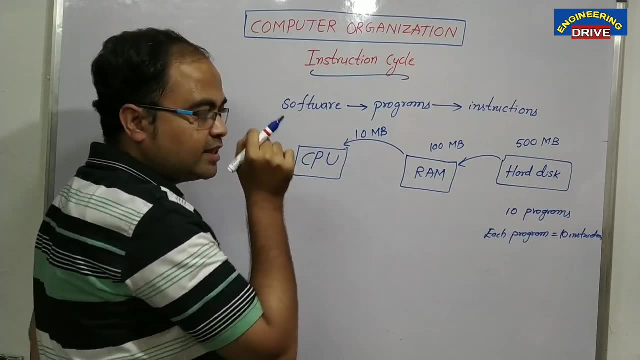 10 instructions my the software which i have installed in my hard disk of 500 mb. it contains 10 programs. again, each program contains how many instructions on an average? let us say 10, which means totally. how many instructions are there in my software now total? 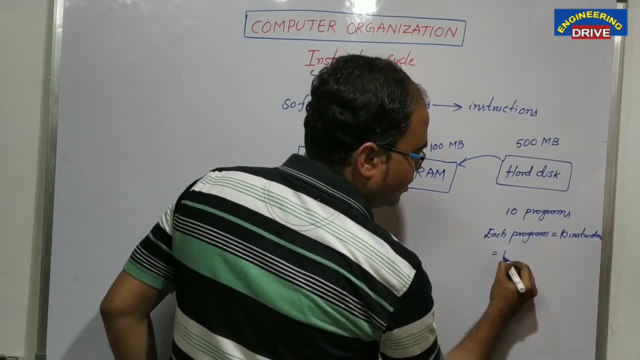 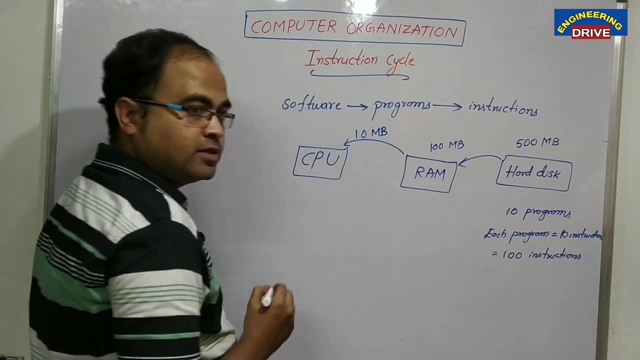 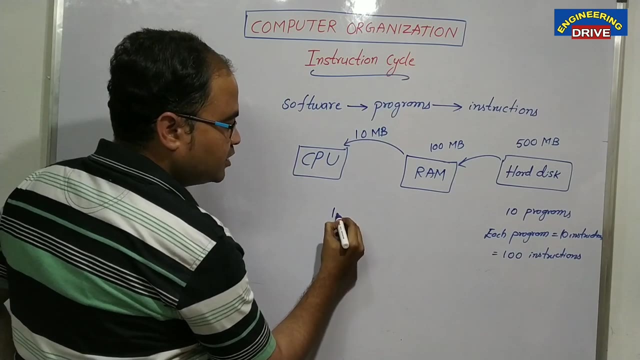 10 into 10. if i combine, if i multiply, then i will get 100 instructions, which means what our cpu will do. now our topic is instruction cycle. what is instruction cycle? first, our cpu will fetch the instruction, that is. this is the first step in our instruction cycle. 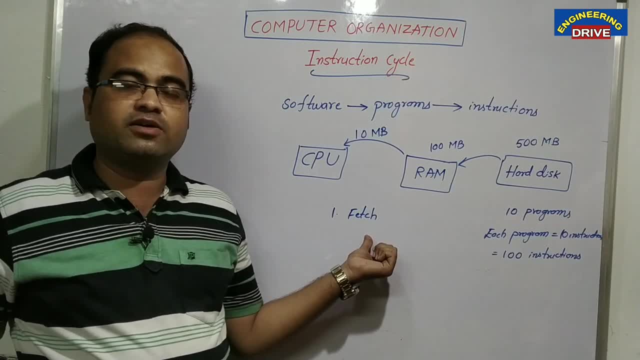 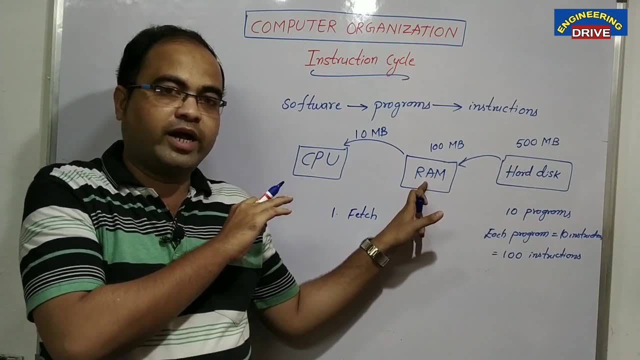 what our cpu will do. it will fetch the instruction. what is meant by fetching the instruction? fetching the instruction means it will take the instruction from hard disk and it is brought into ram from ram. from ram it is copied into cpu and cpu will execute that. okay, fetching is nothing but taking the. 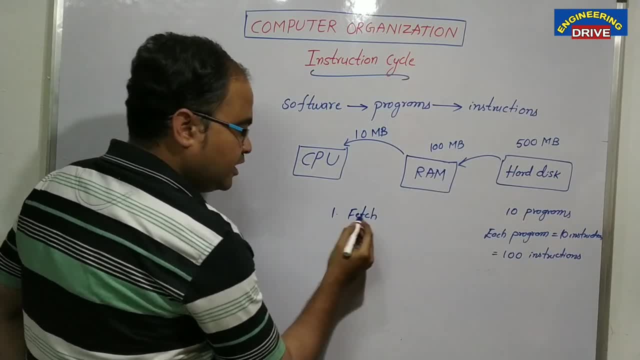 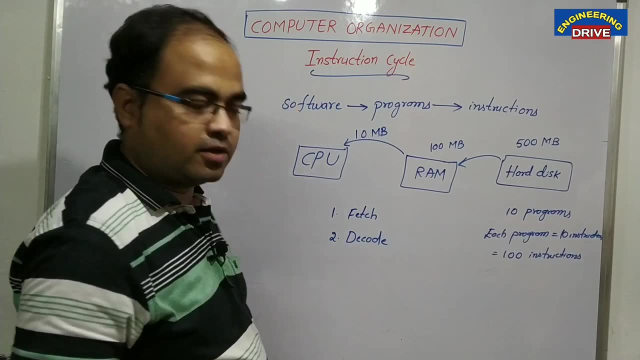 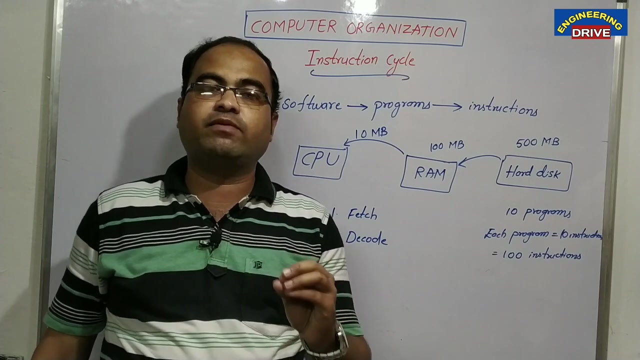 instruction from hard disk or ram to cpu. this is first step and the second step is, in the instruction cycle, decode the instruction. what is it by decoding the instruction? you know our computer understands only one language. the name of the language is machine language or binary language. so decoding the instruction means converting that instruction first. it will fetch the instruction. so 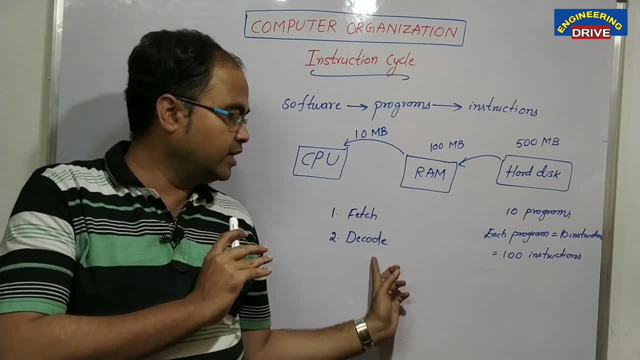 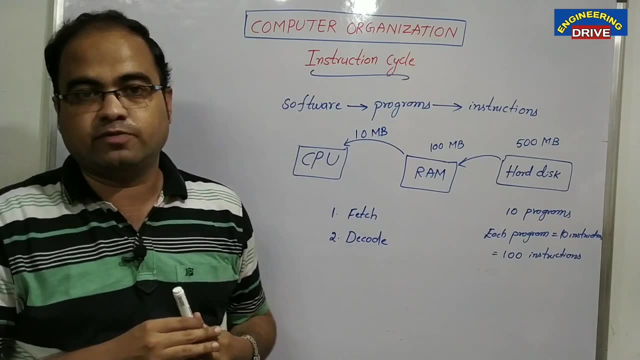 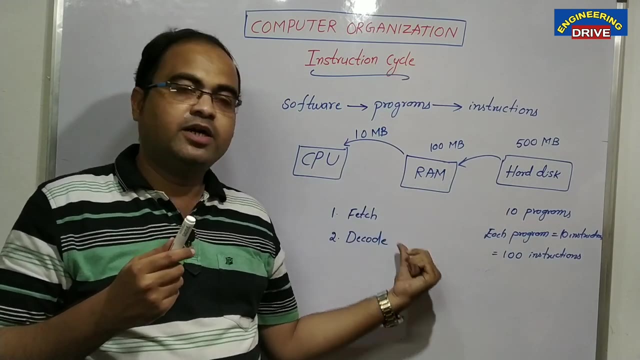 the instruction is there in cpu. okay, fetching completed. second step is decode. decode means our cpu will convert that instruction into binary or machine language. now, okay, the instruction may be in some other language. once the instruction has been copied to cpu- fetching completed. decoding means converting that instruction into appropriate machine language. so conversion will take place in. 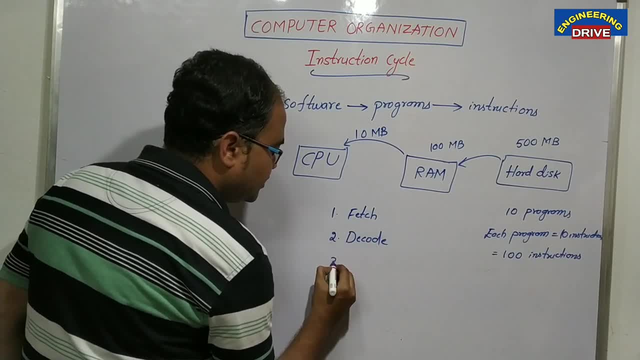 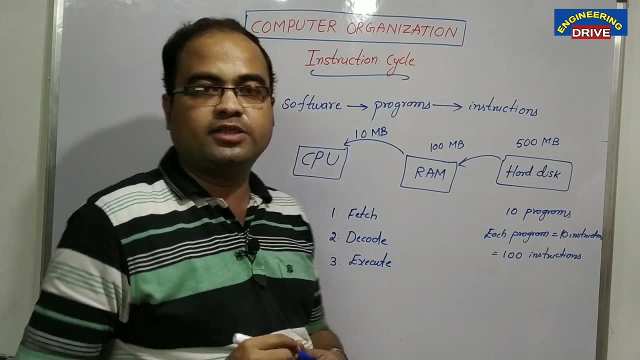 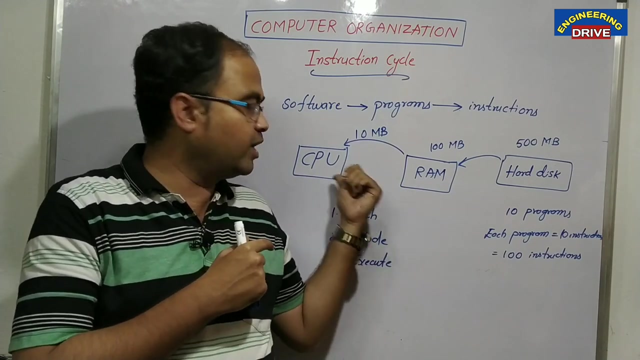 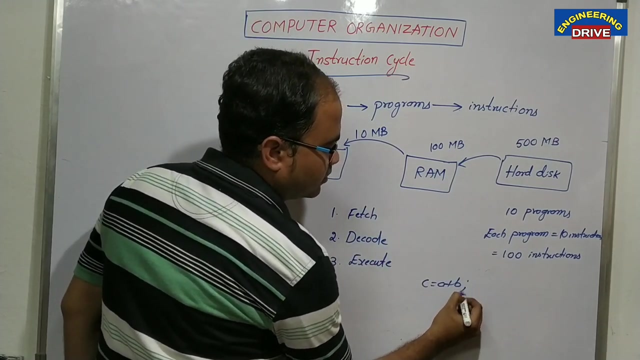 second step, that is decode. and the third step is final step is execute. execute the instruction. what is mean by execute the instruction? whatever the instruction has been for for that work, that work will be completed by cpu. let us say my instruction in our one of my instruction is: c is equal to a plus b. i have written this c language program instruction. 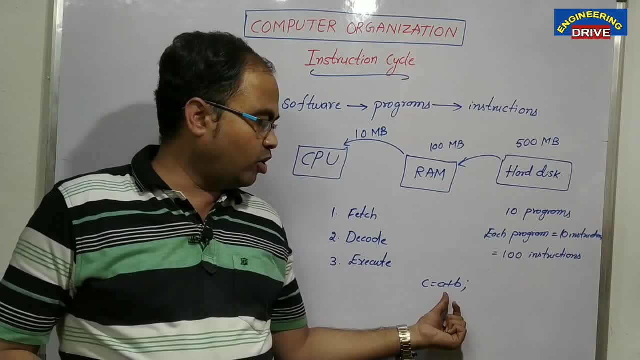 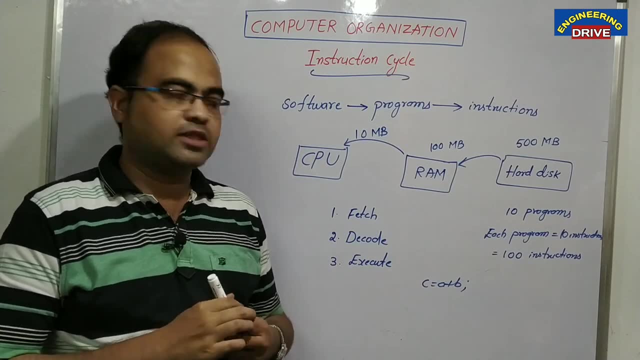 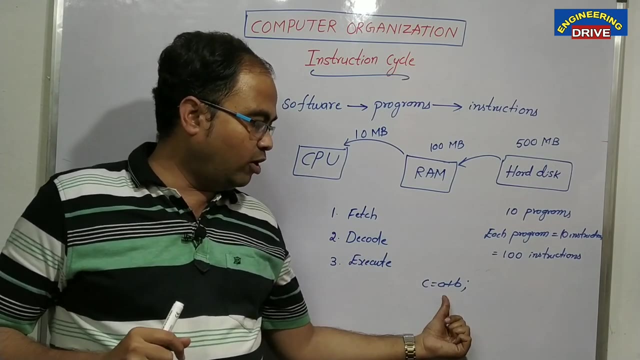 this is one instruction. so what this instruction is doing, it is copying, it is adding the contents of a and b and it is storing the result in c. this is one instruction, okay, so executing the instruction means getting the value of c. how we can get the value of c? the value of a will be added with the value of b. 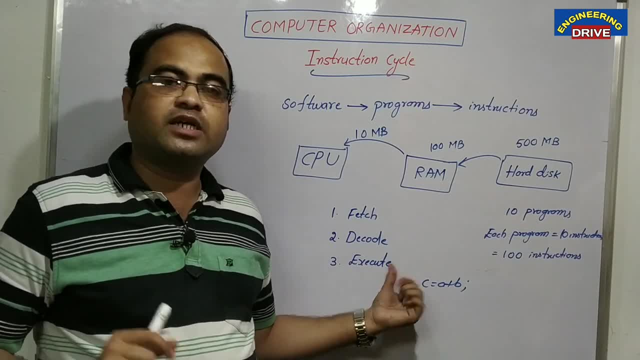 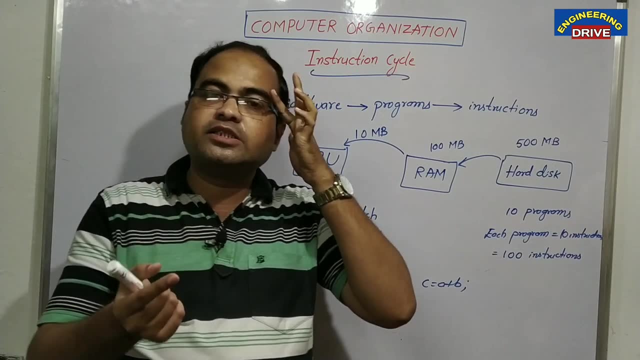 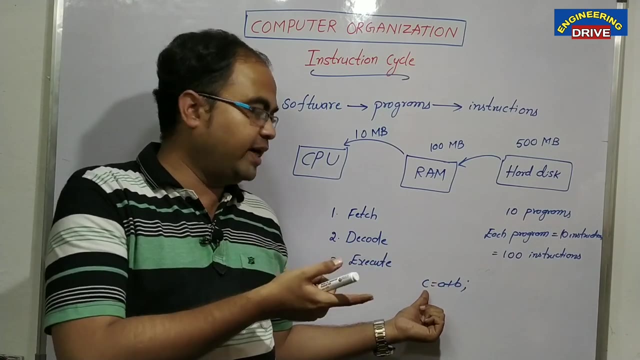 and the result is assigned to c, so which means execution of the instruction has been completed. okay, first step: fetching the instruction. second step, decoding the instruction, which is converting the instruction into appropriate binary language. and the third step is executing the instruction means providing the, or providing that particular desired result. 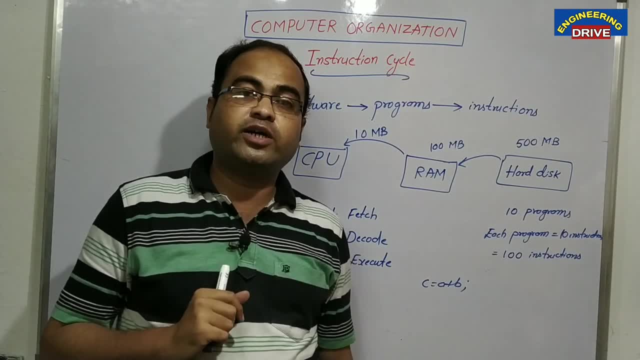 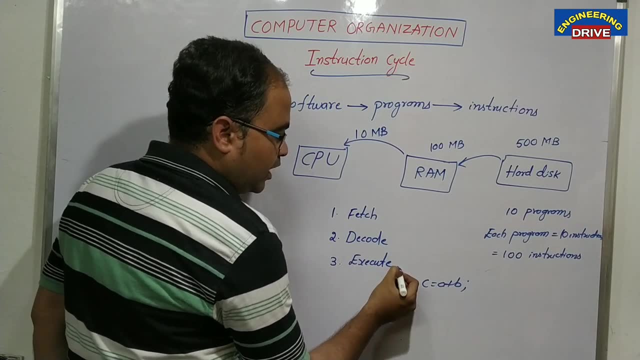 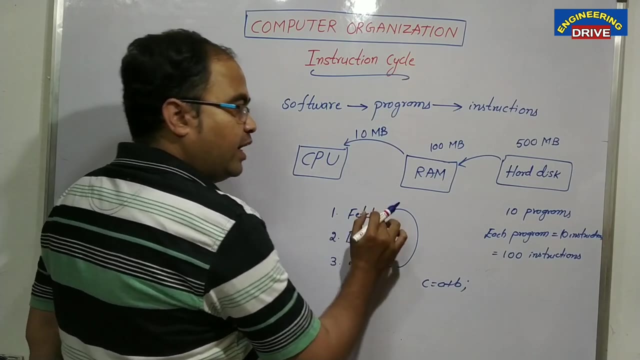 that is, executing the instruction. how many instructions have been executed now? only one instruction has been executed successfully. then what happened again? from here, control will go to the first step. execution of one instruction has been completed. then again, control will go to fetch. then what it will fetch? it won't face the same instruction, it will face the second instruction. 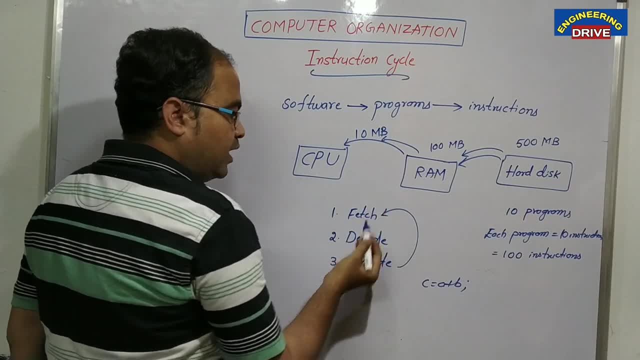 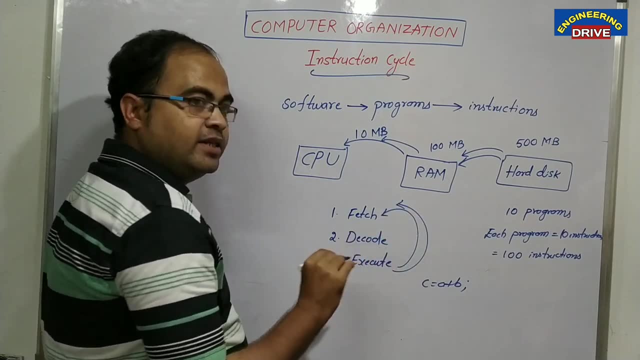 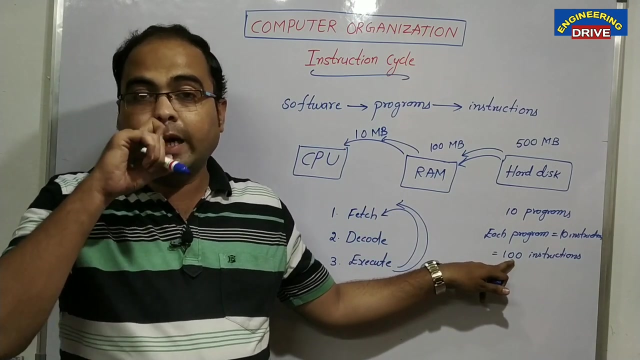 again. second instruction, again second instruction, again decoding of second instruction and then execution of second instruction. again decoding of second instruction and then execution of second instruction, again. the cycle will continue for third time like that. this instruction cycle will repeat how many times? how many times? 100 times. why 100 times? because we are currently running our cpu. 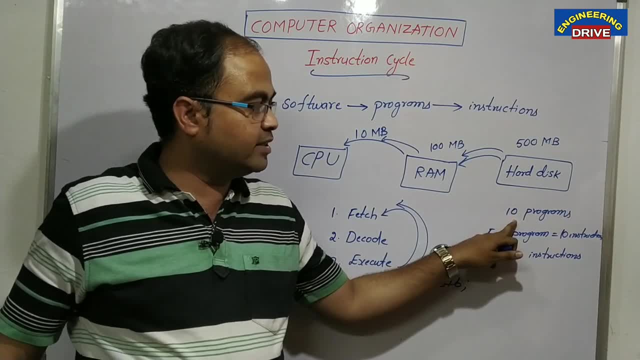 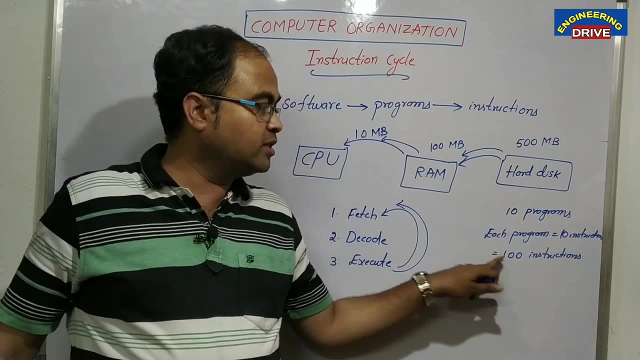 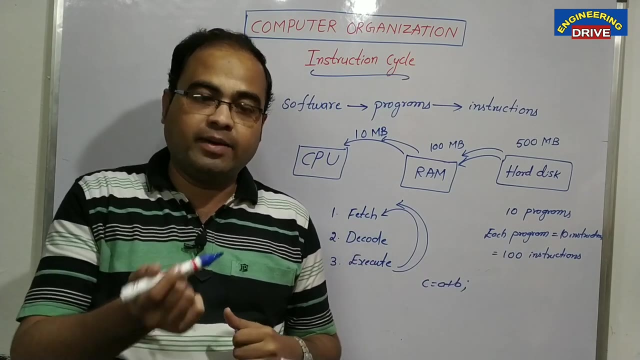 is currently executing a software. in our example we have taken that software that contains how many programs? 10 programs. each program contains how many instructions? 10 instruction, which means our instruction cycle will repeat how many times? 100 times. after 100th time we will get the proper output. that is our final output of the program after. 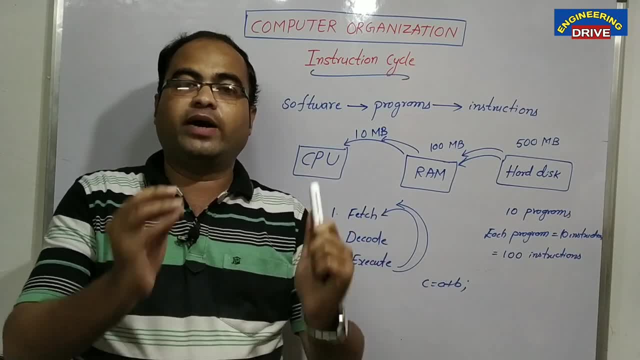 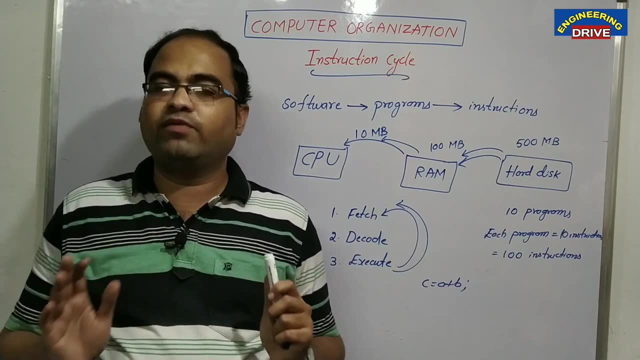 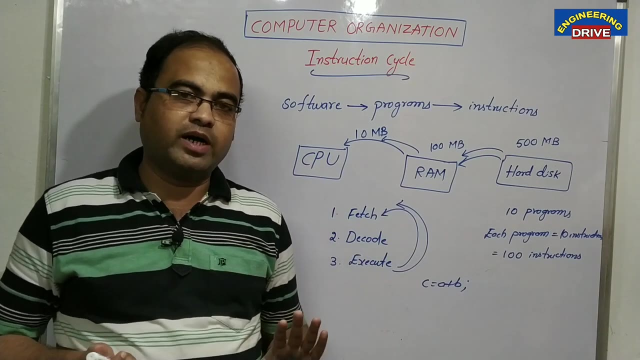 100th instruction is executed, our cpu will provide the desired result. this is our instruction cycle, my dear students. okay, if you, instruction cycle is very, very easy: concept: fetch the instruction, decode the instruction and execute the instruction. if you understand these three steps properly, before understanding this concept, you should know this diagram pretty well, co. if you won't, 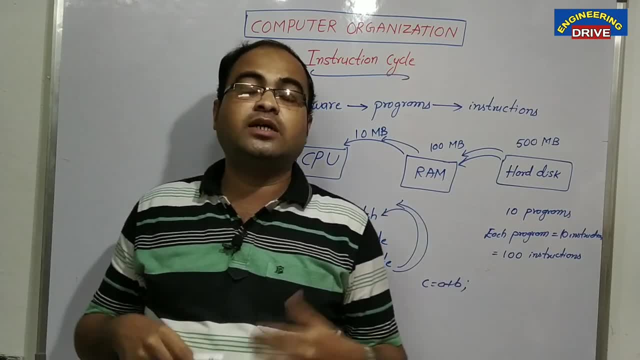 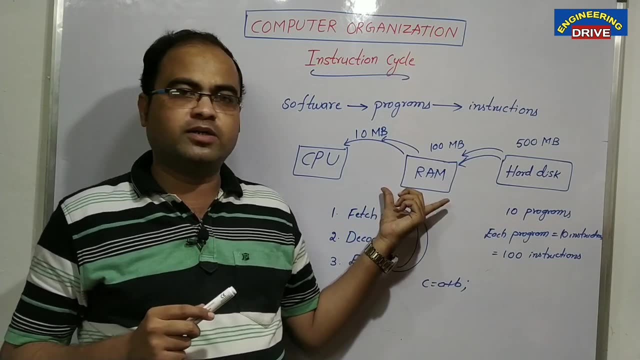 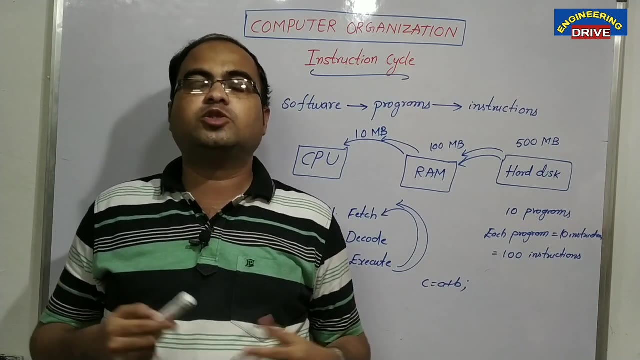 understand this diagram, then it is difficult for you to understand some more concepts in computer organization. first of all that reason, for this reason, you be good in this diagram. first it is simple one. okay, then we can understand easily what is instruction cycle. okay, in competitive exams dash is not a step of instruction cycle. they may give some other step and ask you and dash. 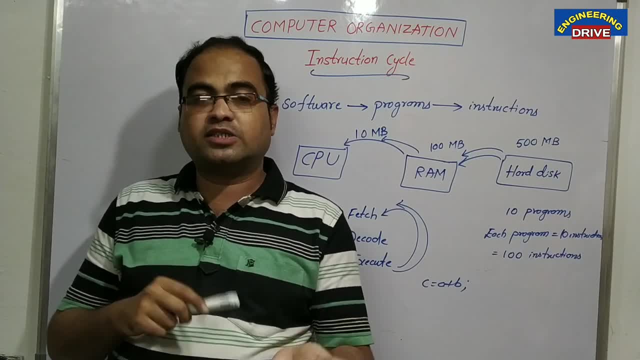 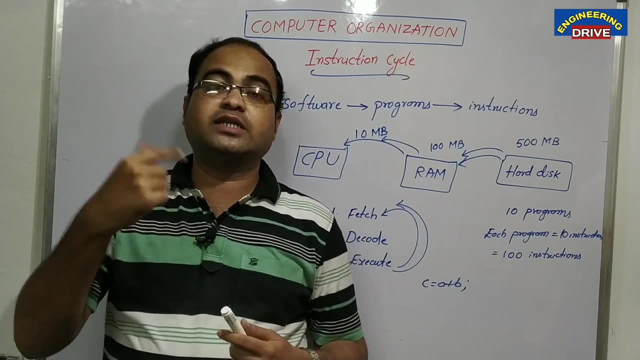 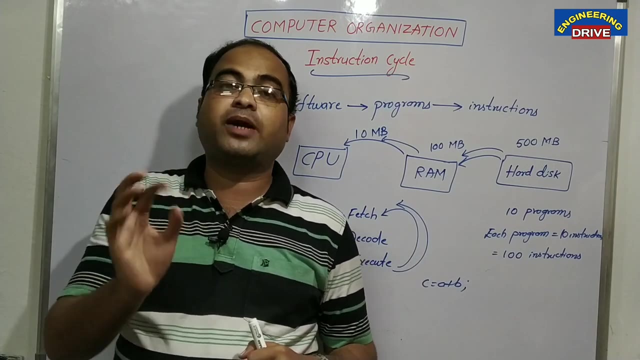 is a step of which converts our instruction into appropriate machine language, then you can write: d dash is a step in instruction cycle by which the result is produced. so when the result will be produced only after execution, step dash is the first and primary step of instruction cycle. 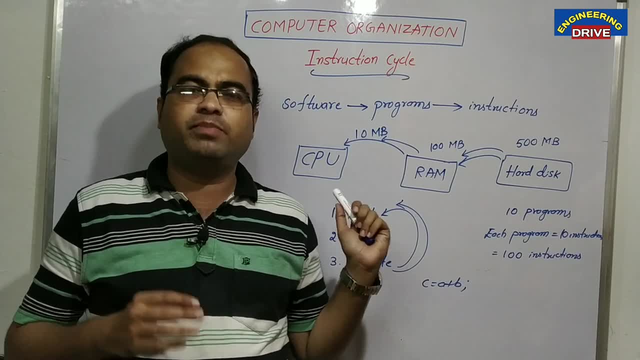 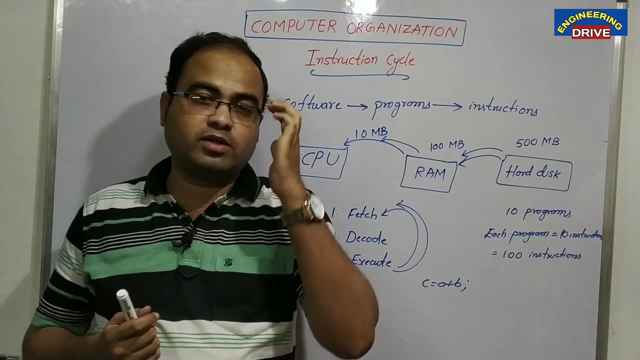 answer is fetch. so these are some of the bits, simple bits that can be asked in the, that can be asked in various competitive exams, and if you go in some more, some more depth, how they can ask the bits you know. let us say our program, let us say we are having 10 programs. 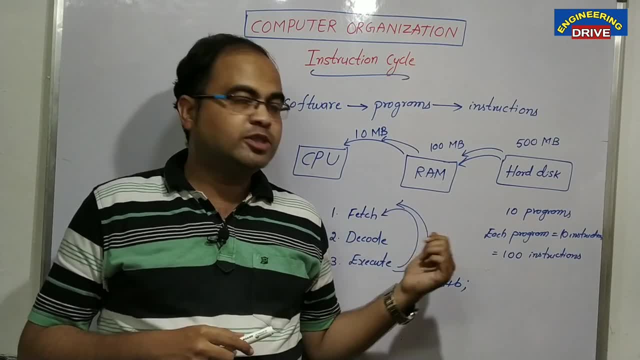 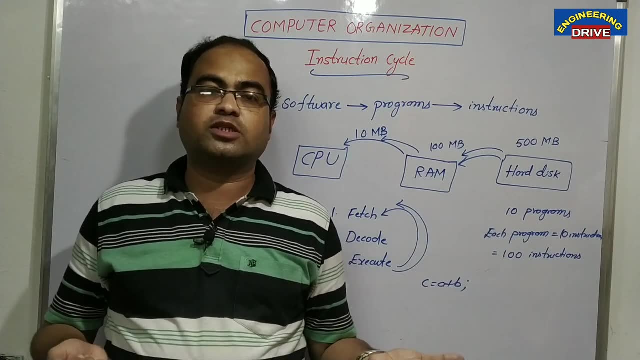 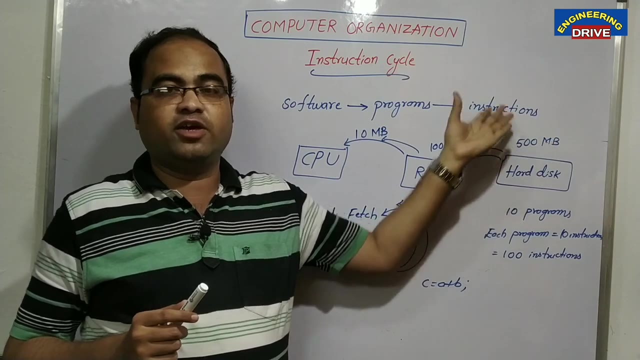 denoted by p and each program contains n instructions, then how many instructions are there in the entire software? they can ask this type of question when you can answer this question. if you know this difference, what is a software? what is program? what is instruction? if you know, 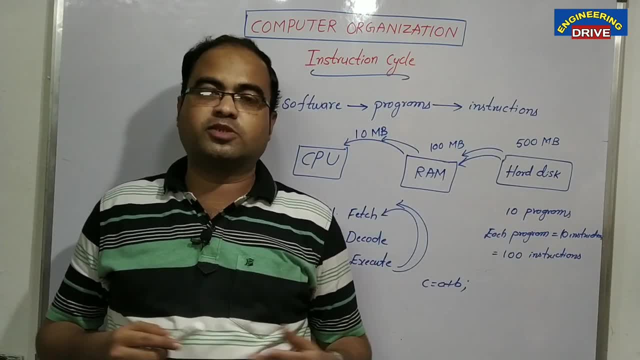 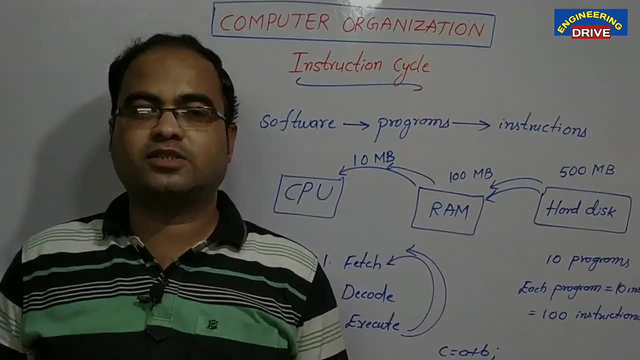 this properly, easily, you can able to solve this, those type of problems also, okay. so with this, let us close this today's session of video. see you soon. take care. love is you. 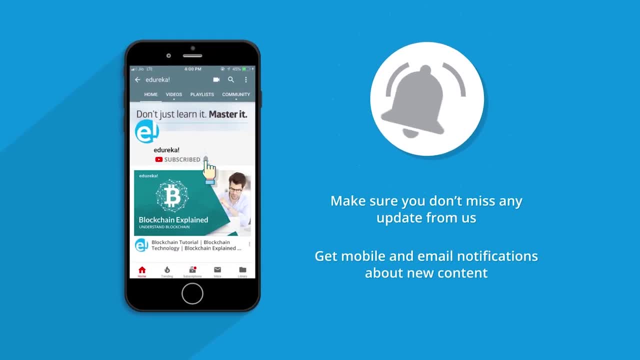 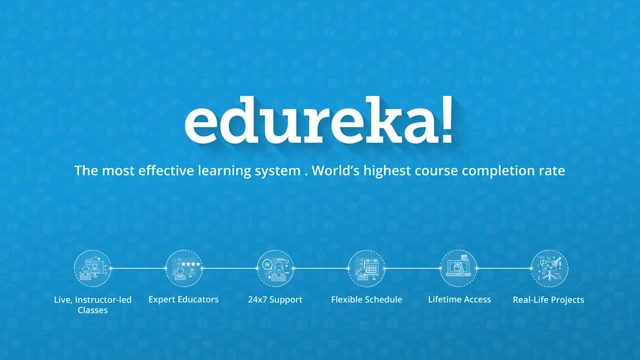 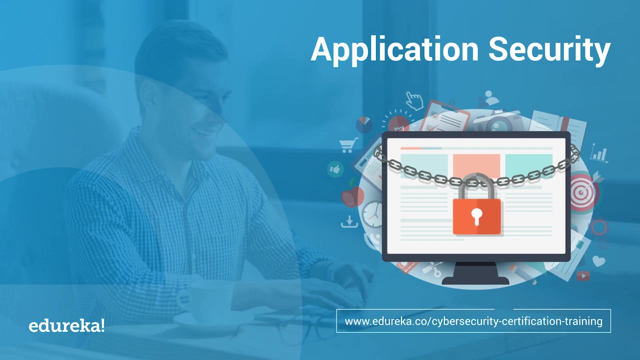 Cyberspace continues to transform the way we live and the way we do business. Securing cyberspace has become a critical need in 21st century to enable people, enterprises and government to interact and conduct their business. Hey guys, I'm Archana from Edureka and I welcome you to this session on application. 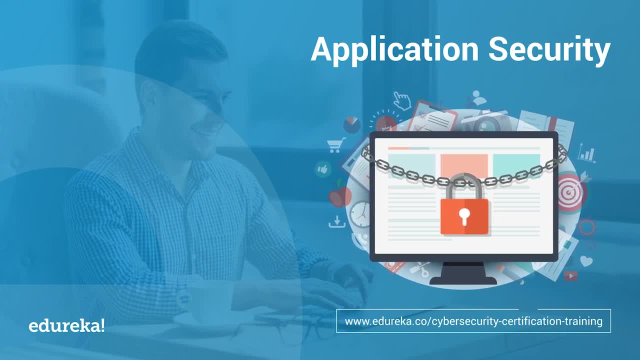 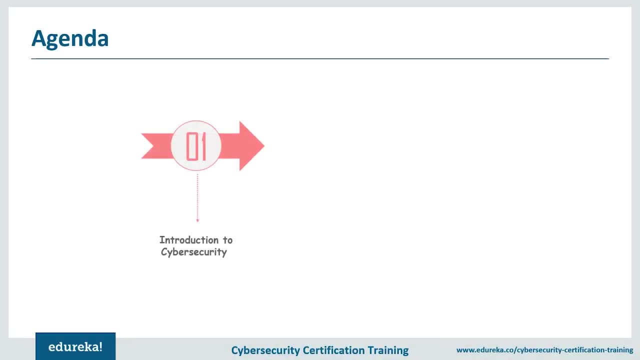 security. So, without any delay, let's take a look at topics that we will be talking about today. We will begin by discussing what cyber security is and why it is necessary. Then we'll take a look at what application security is and why applications seems to be great. 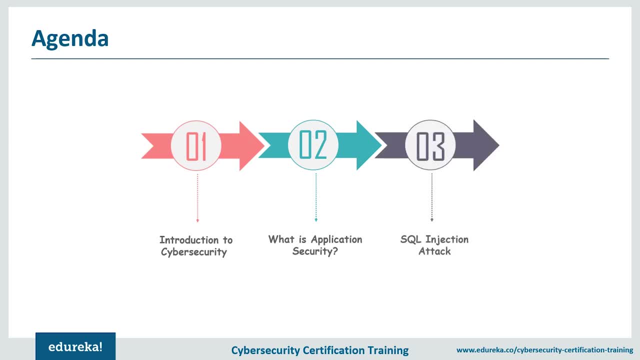 target for cyber crimes. And finally, we'll see what SQL injection attack is and how to perform one on an vulnerable application in the demo part of the session. So I hope agenda was clear to you guys. Let's get started then. Today, our entire modern way of life, from communication to e-commerce, fundamentally 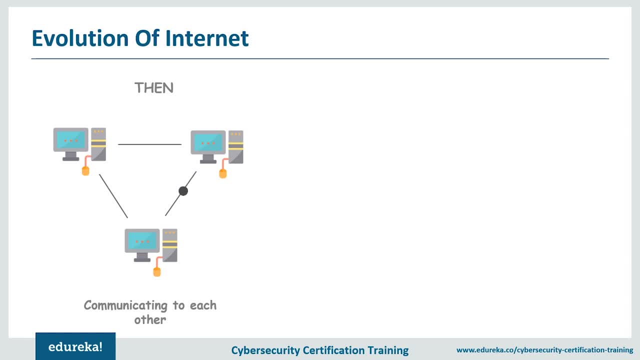 depends on internet. Internet was not originally built to be what it is today. Internet originally developed when computers were so huge and so expensive that only few organizations and government had them. The purpose of internet then was to create a system that would be able to perform one.